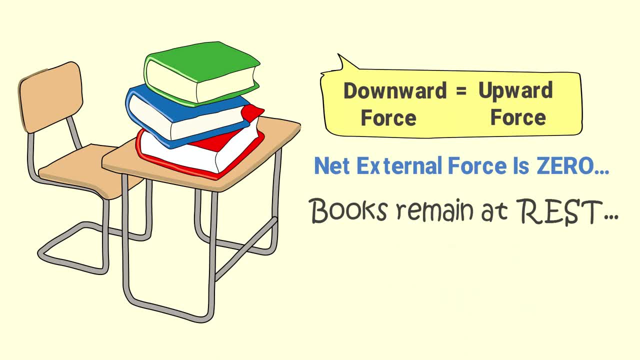 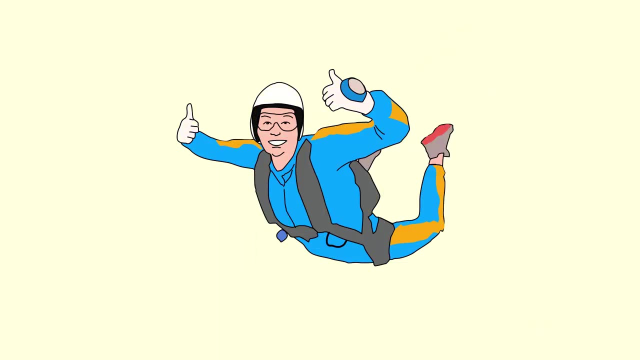 usually call and teach to my students that Newton's first law of motion is also known as a law of balanced forces. Now the second application of Newton's first law of motion is the jumping or free fall of paratrooper. When paratrooper jump off, initially the downward. 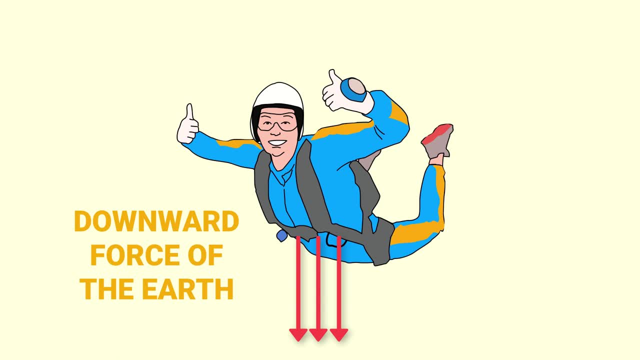 force of gravity on the paratrooper is very high. Hence this downward force provides reduced acceleration in this paratrooper. As a result, the paratrooper accelerates towards the earth center, But at the same time this paratrooper experiences an upward force of. 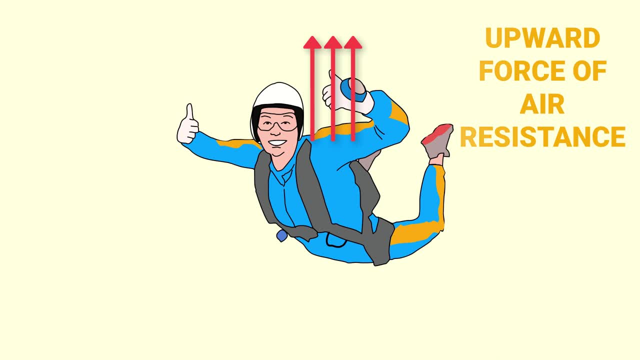 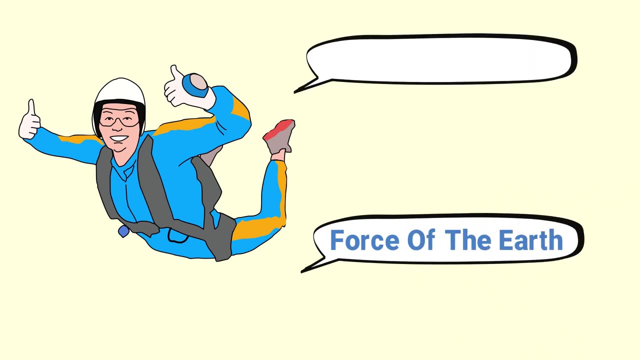 air resistance or air friction. Now, this paratrooper is under the action of two forces: the downward force of the earth and the air resistance. But the downward force of the earth is greater than the air resistance, Due to which this paratrooper accelerates towards the center. 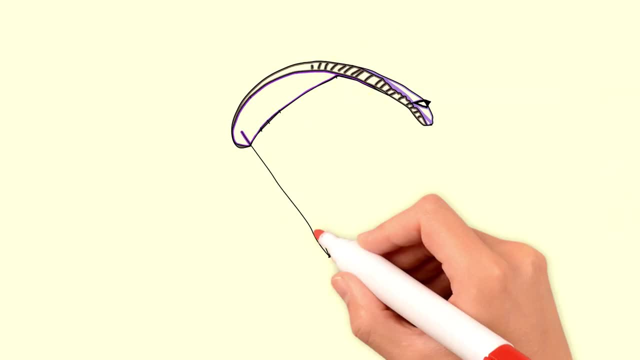 of the earth. When this paratrooper opens the parachute, something interesting happens. This parachute increases the surface area for this paratrooper. Thus the air resistance on the paratrooper becomes increasing as the paratrooper falls towards the earth. A time. 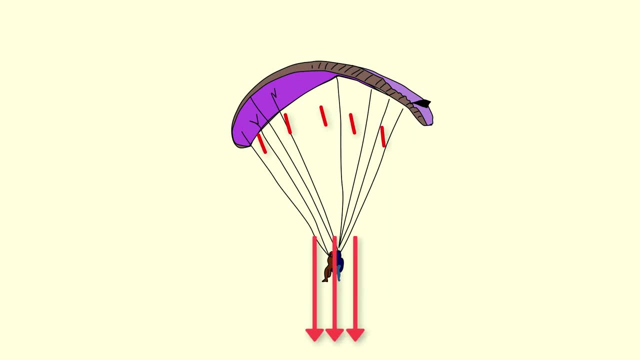 comes when the downward force of gravity on the paratrooper increases. Thus the downward force of the earth and the upward force of the air, or air resistance, becomes equal. As a result, paratrooper starts falling with uniform velocity towards the earth and execute. 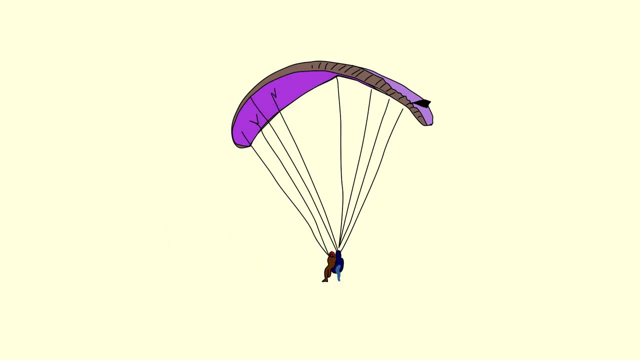 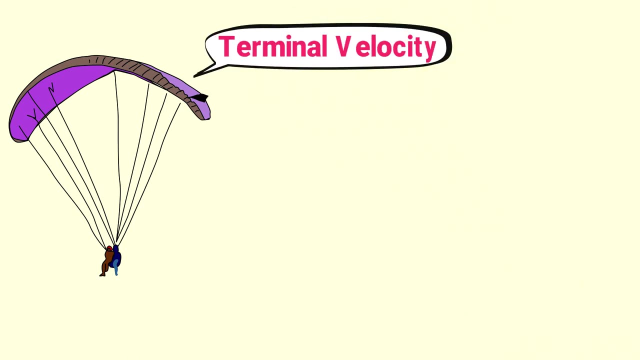 its journey safely. Remember that the uniform velocity of the paratrooper is also known as a terminal velocity. Now here comes the most interesting and difficult question of this lecture. When the downward force or the upward force on the paratrooper becomes equal, then why this paratrooper doesn't stay up in the air, or why this paratrooper doesn't? 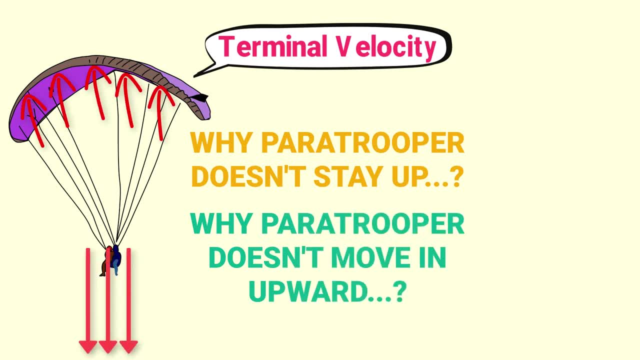 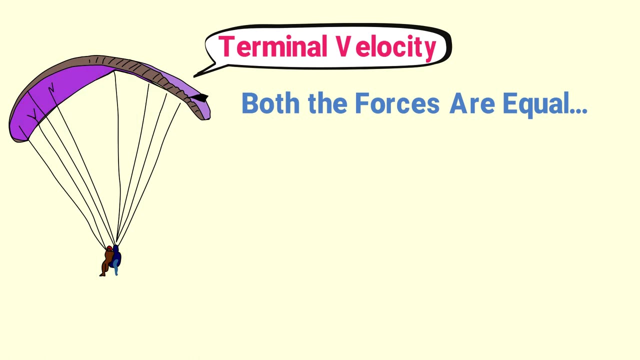 move in upward direction Because both the downward force and the upward force are equal. Can you guess the answer? Let me explain it for you, As we know that both the forces are the paratrooper, but the paratrooper falls downward. it is due to inertia. now, 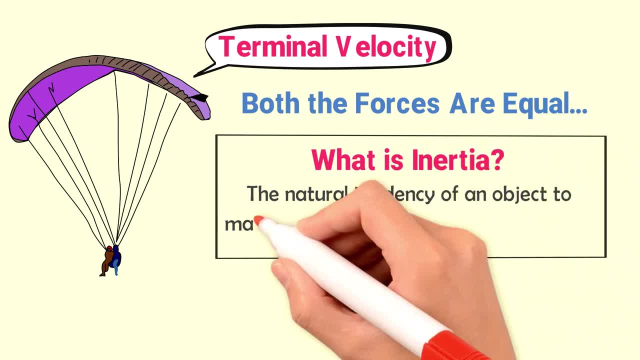 what is inertia? inertia is the natural tendency of an object to maintain its initial state of rest, our initial state of uniform motion. here, initially, the paratrooper was in motion and downward direction. when the downward force and upward force becomes equal, here appears the black ghost of inertia and it tells: 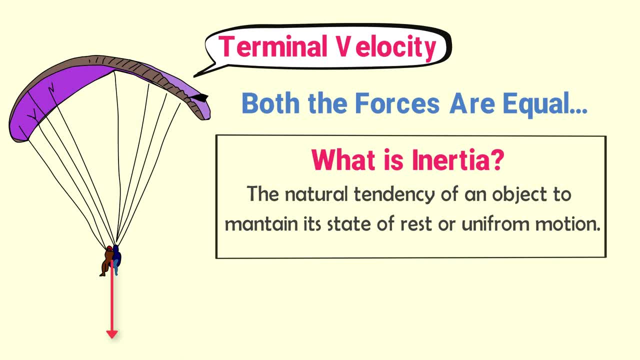 the paratrooper. initially you were in downward motion, so again you have to be in downward motion. therefore, this poor paratroopers fall with terminal velocity and downward direction due to inertia. the third application of Newton's first law of motion in our daily life is the law of motion. 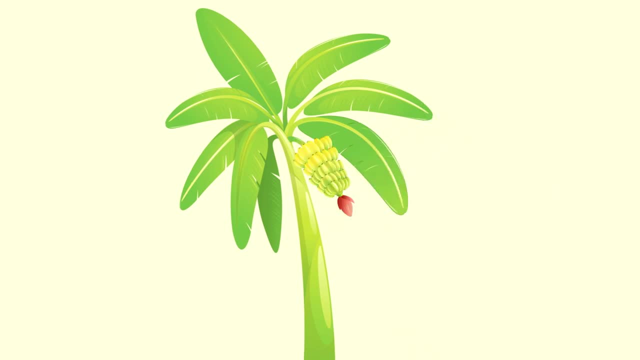 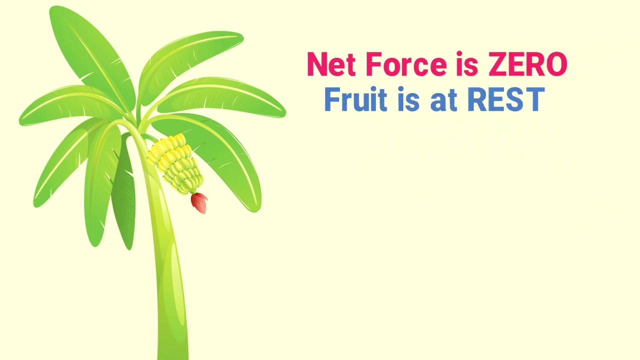 in our daily life is falling of fruits from any tree. when you shake a tree, usually fruits fall down the tree initially. this fruit is it rest because the downward force of the earth and the upward force of leaf stick is equal. thus net external force on this fruit is zero. that's why this fruit is it rest, the 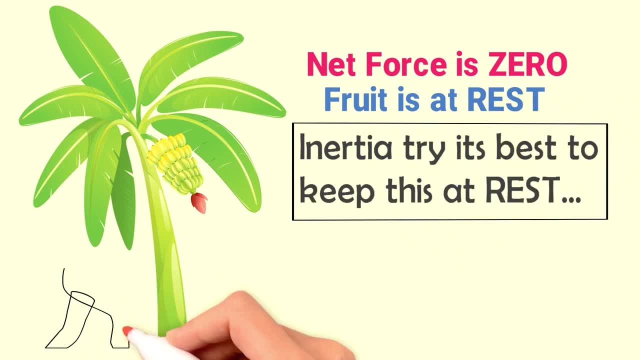 inertia of this fruit will try its best to maintain its normal state of rest. it will rest until to keep this fruit at rest. now, when you shake the tree, this will disturb the net external force on this fruit. are the net external force wouldn't be equal. hence, 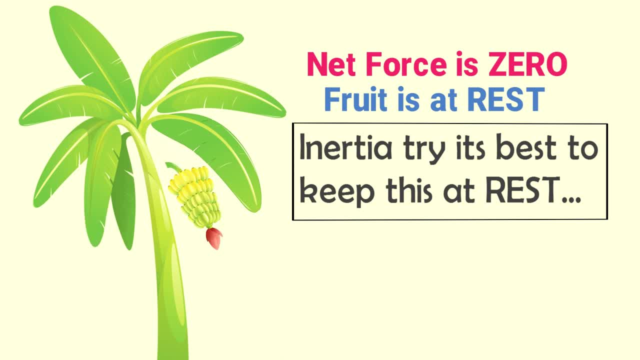 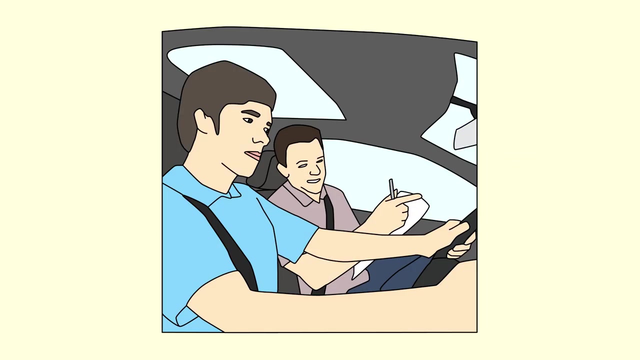 the fruit will be separated from the tree and it will stay here because of inertia. now here comes another force, our downward force of the earth, which pulls down this fruit towards the earth center and it falls down. lastly, when you travel in a car, in your car suddenly apply a break, you feel a forward, jerk, a forward.